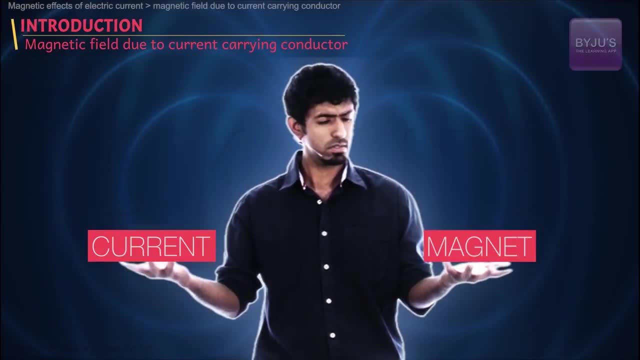 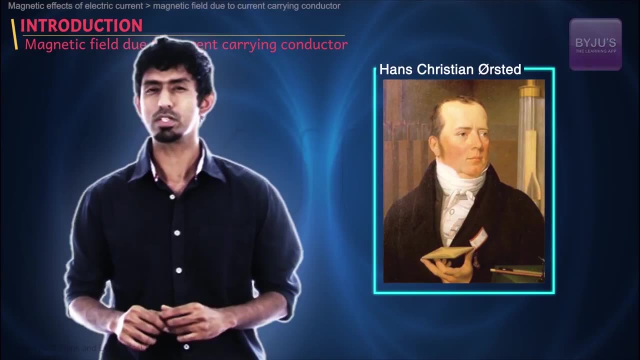 So we know current separately and we know magnet separately, Not so connected Till. one man called Oysted in a lecture noticed something extremely fascinating. He noticed that there was a current carrying conductor right. We all know what this is: a wire with some current going. 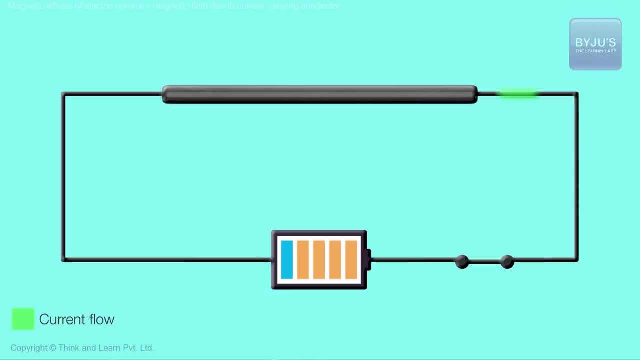 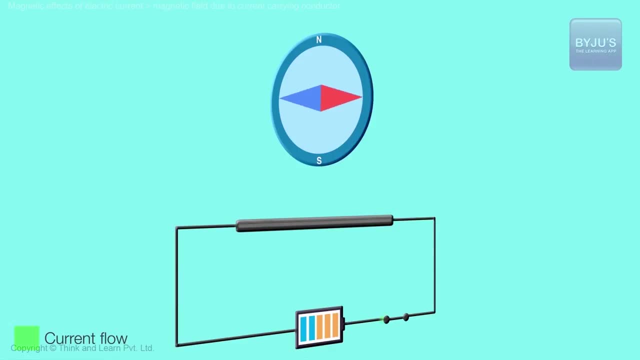 through it, Put it across a battery. there'll be some current. This we've done in the previous chapter. All of a sudden, he noticed that the compass needle next to this wire started to turn, and that was not expected, And we all know that this happens. When does it happen? When does the 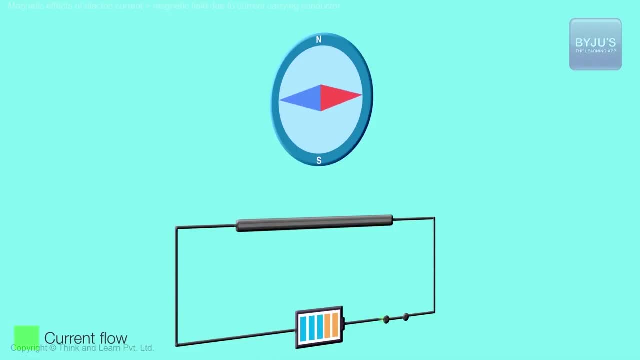 compass needle start deflecting from its original position? Yes, when you take a bar magnet next to it, right, But there is no bar magnet here. There is a wire carrying current and this magnetic compass is beginning to turn next to that wire. So this was very fascinating and he started playing. 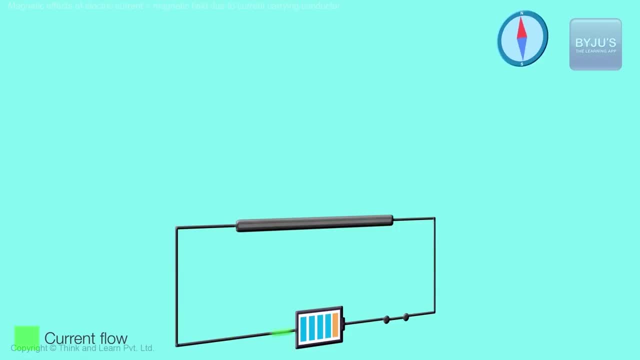 with this. He started taking further and further away. The effect wasn't much. He brought it closer and closer. It started turning more. Then he switched off the power and all of a sudden it went back to the old position it pointed, Which is north and south, as it always does Now. this was very fascinating, He began to realize. 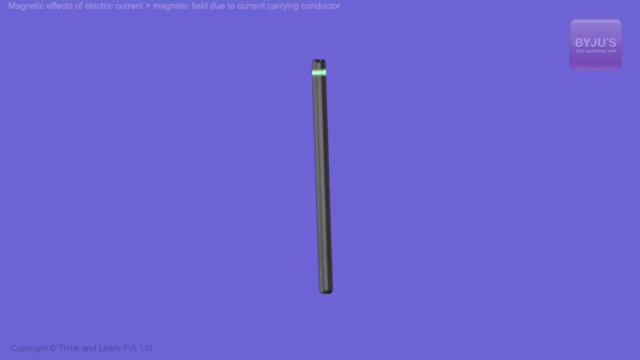 something very, very important. What was that? Somehow a current carrying conductor was behaving just like a magnet would. That's fascinating, because we thought these two are separate. It was a moment, just like Newton, realized, when the apple that falls down is the same thing as 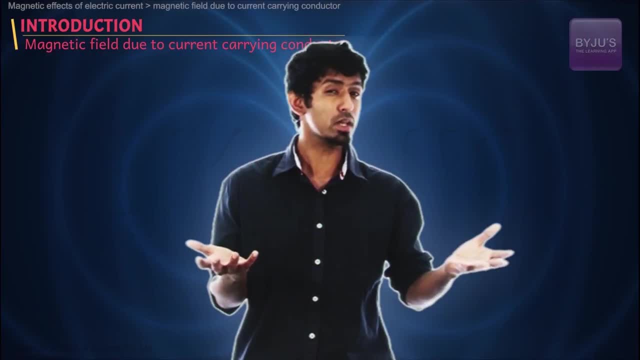 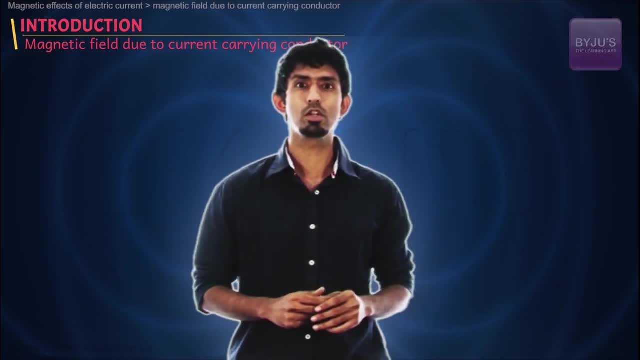 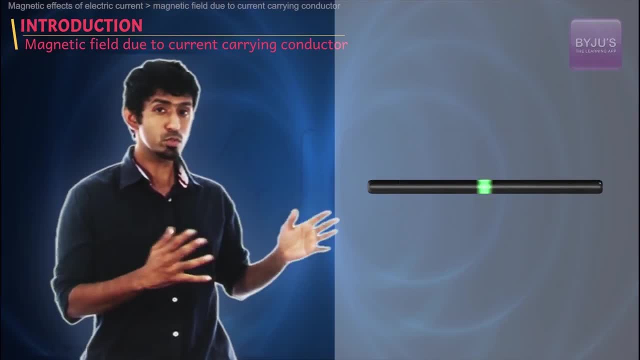 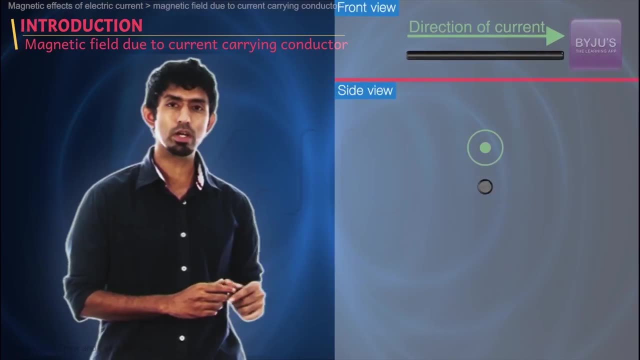 you know there are some charges going through it. We all know that they're going in some direction, So we would say: the current is flowing in that particular direction. Imaginary positive charges. If that were true, then if I were to turn this wire this way, such that the wire is coming right, 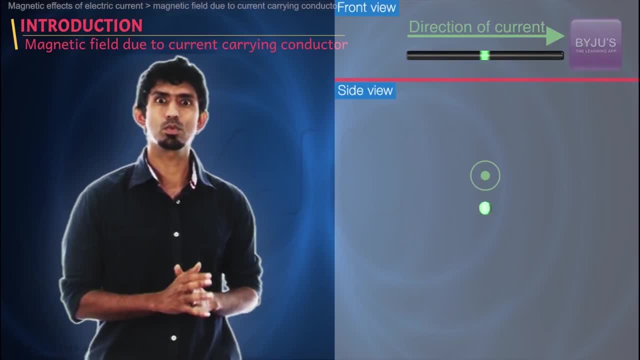 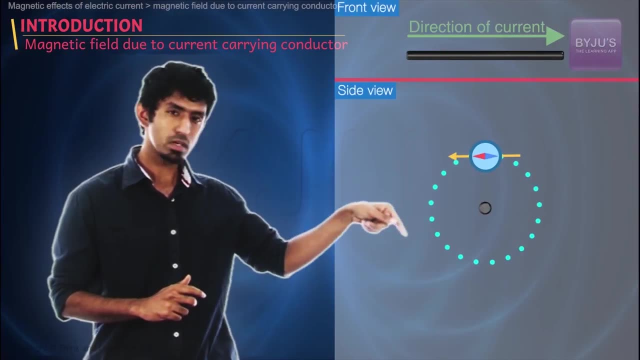 at you, with the current flowing right at you, then let's imagine what would happen If I were to take a compass and keep it. in various points. he found something very, very fascinating: That the compass points in a direction that's tangential to an imaginary circle, And that means